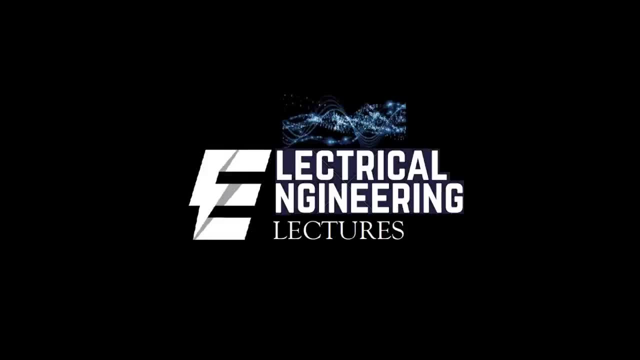 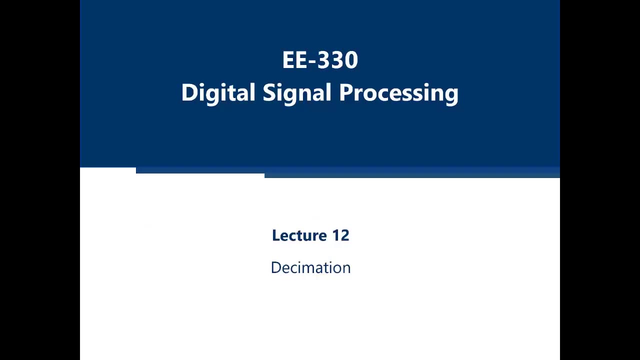 Hi viewers, welcome to our electrical engineering lecture channel for most interactive sessions of different subjects of electronic and electrical engineering. For the latest updates and videos, don't forget to subscribe and click the like button. Assalamu alaikum everyone. In today's lecture of digital signal processing, we will be discussing 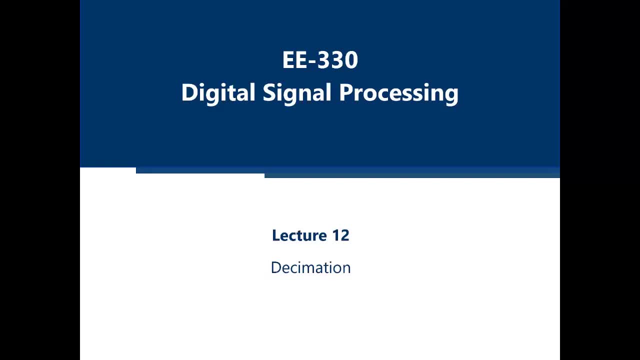 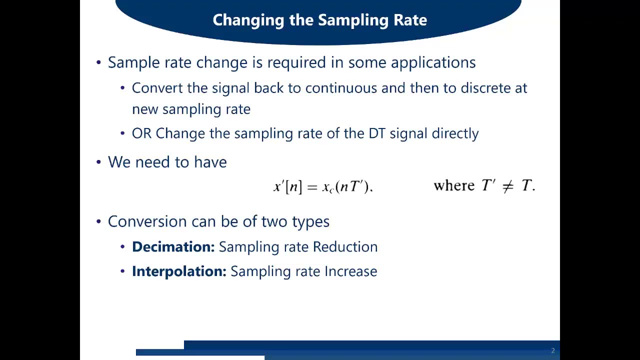 the concept of sampling rate change and, in particular, the concept of decimation or downsampling. Why sampling rate change is required? in case of practical systems, Sampling rate change means either we need to decrease the sampling rate or we need to increase the sampling rate. 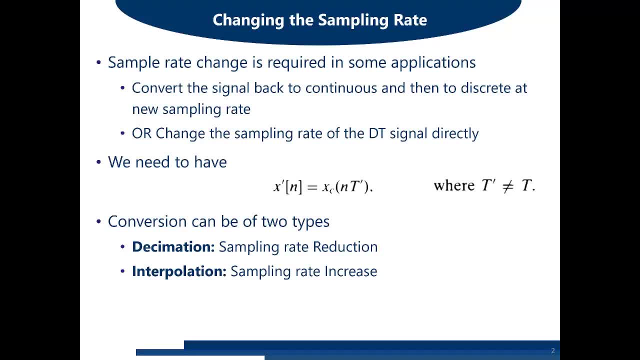 Why we need to decrease the sampling rate. Because in some practical systems, due to some hardware constraints and availability of resources, we cannot process the discrete time sequence in its original form. So we need to reduce the number of samples and that is called reducing the sampling rate. 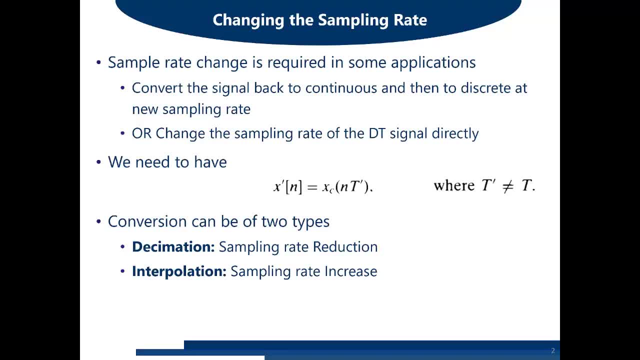 And in particular in digital image processing or similar applications, there are cases in which we want to increase the sampling rate. So now, this sampling rate change can be achieved by either of two ways. The first one will be, that is, to convert the signal back to continuous and then again perform. 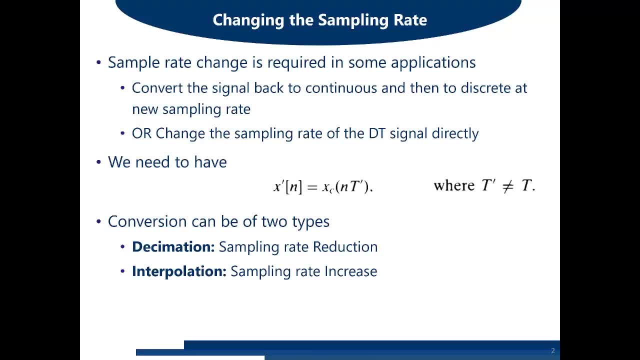 the sampling at a new sampling rate, And the second option will be to change the sampling rate of the discrete time signal directly. So the concept is that we have x of n or any discrete time sequence in hand. So the first option will be to convert this x of n into continuous form and then 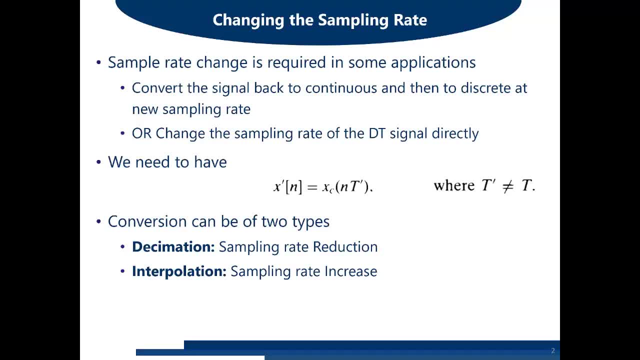 again perform the periodic sampling or any kind of sampling at a new sampling rate. But that option is not definitely desired because it involves two stages. Number one is reconstruction and number two is resampling. So the second option is more practical and more easy because 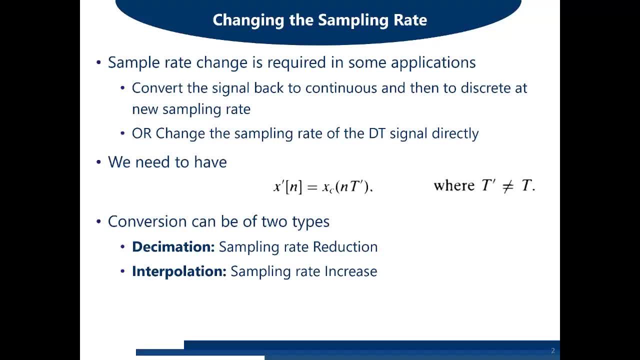 it requires the sampling rate change directly, without going into the reconstruction or sampling stage. so now, what is the basic requirement that we need to have now new X dash of n, which will be X, C of NT bar and T prime. and this T prime is not. 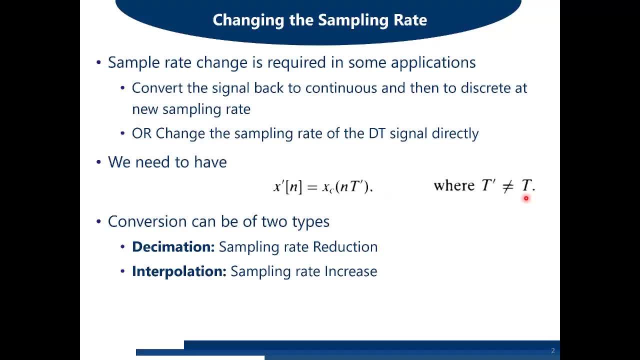 equal to capital T, which was the original sampling period. so it means now we need to have X of n, X prime of n, which is sampled at a new sampling rate, sampling period, T prime. so conversion can be of two types, as I have already told you. number one is decimation, which is sampling rate, reduction or sampling. 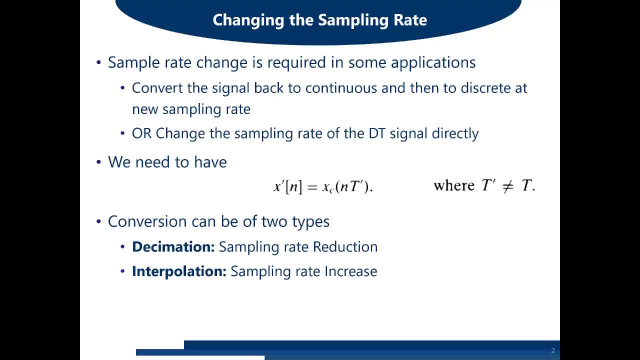 rate decrease and the second one is interpolation, which is sampling rate increase. in this lecture we will be discussing at the concept of decimation and in the coming lectures we will be discussing interpolation. so sampling rate reduction by an integer factor. point number one that should be that 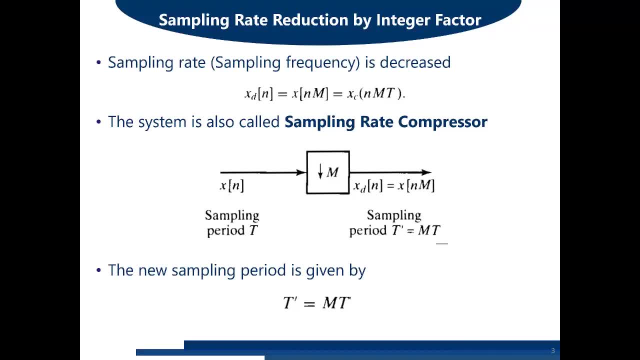 must be kept in mind is whenever we talk about decimation or downsampling, it will be achieved only through an integer factor: you. so what does that mean? it means that the downsampled or decimated signal, now X, D of n, that will be equal to X of n, capital M, where capital M is the 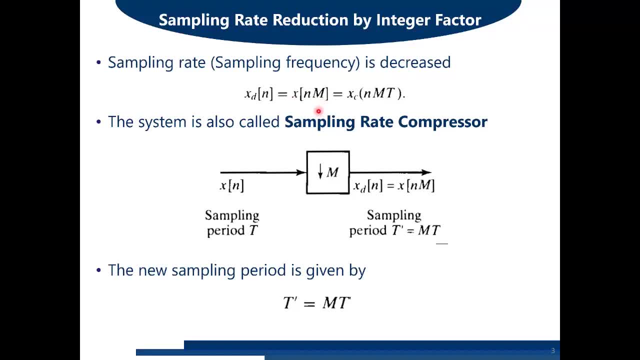 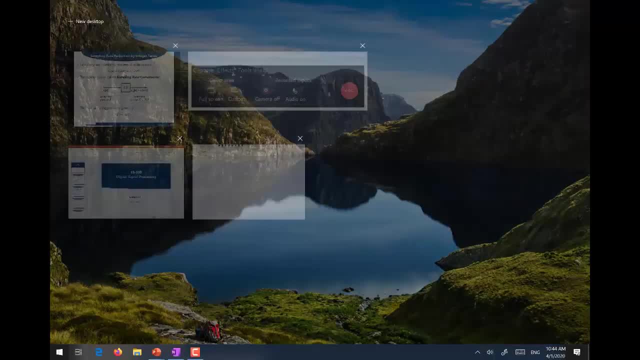 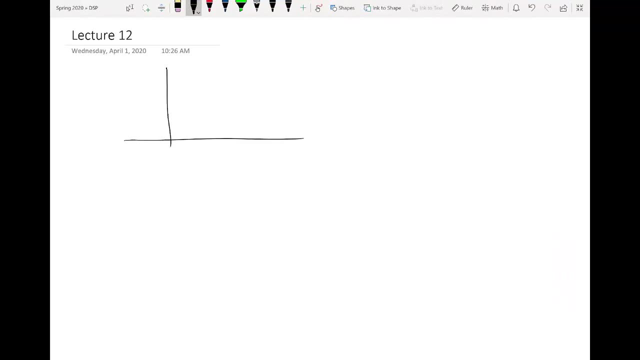 integer or it is a number, which is which describes us that how we need to decimate our signal. to just have a glimpse of that equation graphically, let me draw a discrete time signal X of n, for example. it looks like this: here it is M starting from 0, 1, 2, 3, 4 and 5, and let's say it is 0 at the other values of n you. 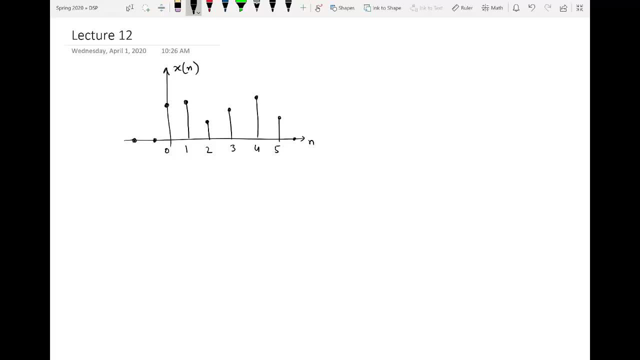 can assume any values of the amplitude. we are not concerned in the amplitudes in this particular case. so now, what we are trying to do? we're trying to find a interrupt right here. we are trying to decimate the signal. it means we are going to reduce the sampling frequency. sampling frequency: let us denote it by FS. 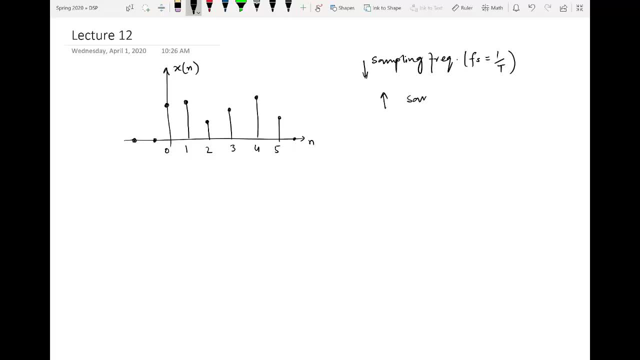 and you should know that this is 1 over capital TV or capital T is the sampling period. it means we are going to increase the sampling period. so point number one that should be kept in mind is that whenever we talk about destination, so we are rate- These are both the same things, But it will mean that 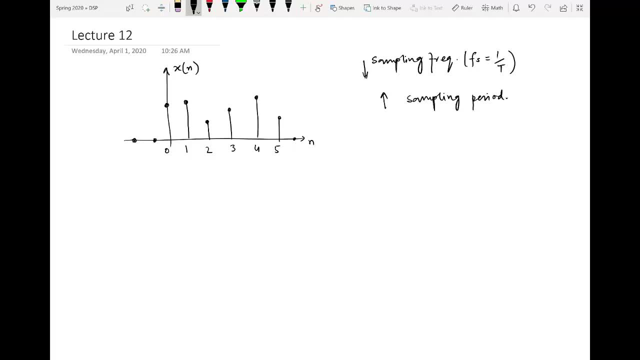 we are going to increase the sampling period because both are inverse or reciprocal of each other. So that factor of decimation, or decimation factor, is denoted by capital M, Decimation or downsampling factor, and it will always be integer. So let's say we are going to set a value. 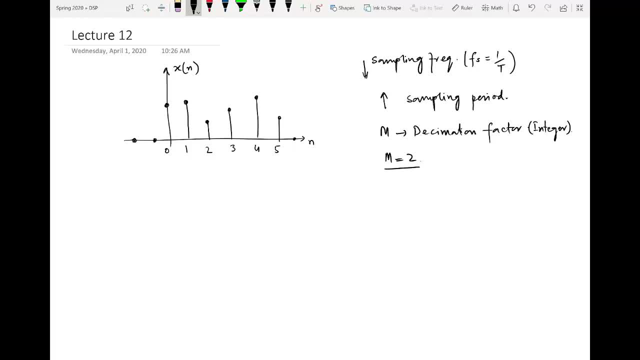 of M is equal to 2.. So we are performing decimation by a factor of 2.. What does it mean? It will mean that we are increasing the sampling rate or reducing the sampling period, which will mean that we are going to compress the signal. 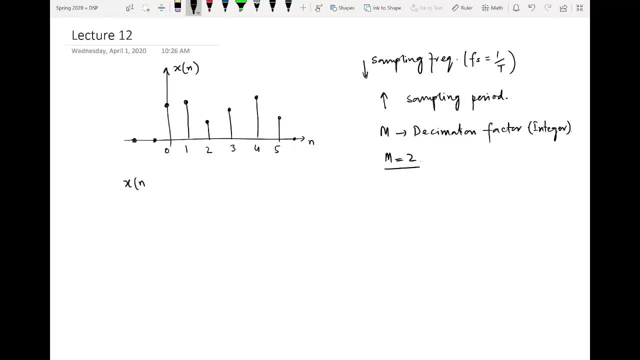 Because the equation that we have shown, that you have just seen in the slide, it was stating that xD of n will be equal to x of nM. So we are actually multiplying the argument of x of n with a number which is greater than 1.. 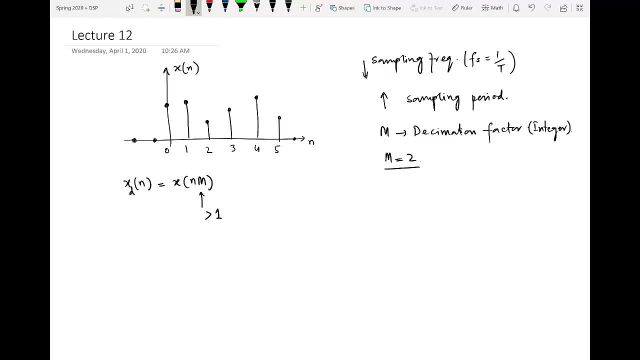 It means we are compressing the signal, because whenever we multiply a discrete time signal or any continuous time signal, we multiply the time with a number which is greater than 1.. It means we are going to compress the signal. So here we are going to multiply it by 2.. 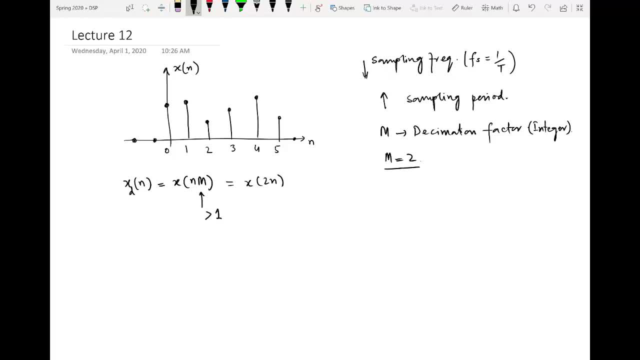 So it means we are going to compress it by a factor of 2.. What does it mean? It will mean that we will discard M minus 1 samples after every sample. M minus 1 sample after every sample. So it will mean that we will keep. 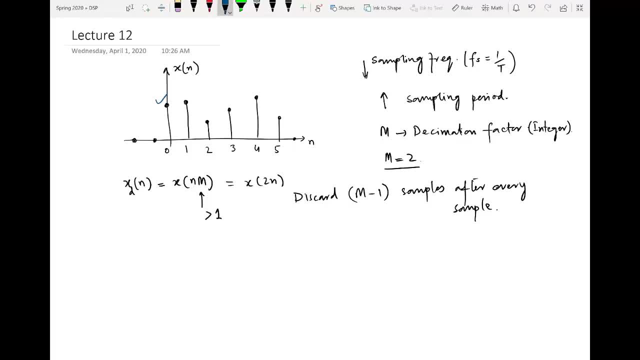 the first one, we will keep this one, we will keep this one, we will keep this one and we will discard the alternate ones. So, when we discard the alternate ones, the new signal, which is xD of n, xD of n, it will only 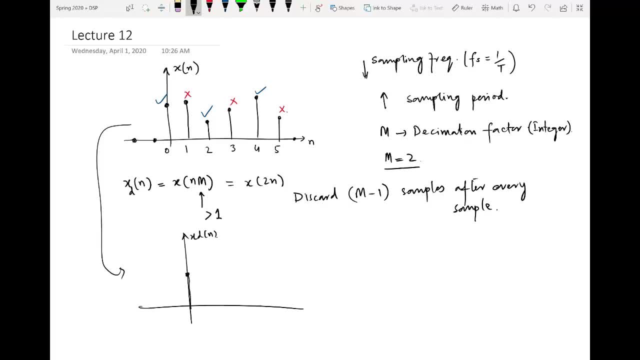 contain 3 samples and not 6 samples. This is the first one, it will be the second one and it will be the third one. There will be a slight change in the amplitudes, just because I am drawing a rough sketch: 0,, 1, 2 and others will be 0. 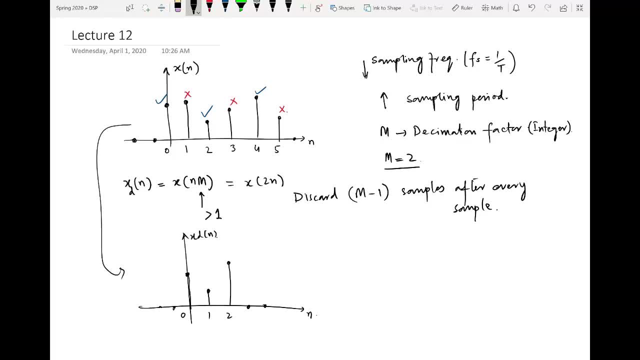 So now you see, the time domain signal is compressed due to the multiplication of a factor of 2 within the argument of the signal. So you see, instead of having 6 samples now we are having 3 samples, and that is intuitively describing us that we are actually. 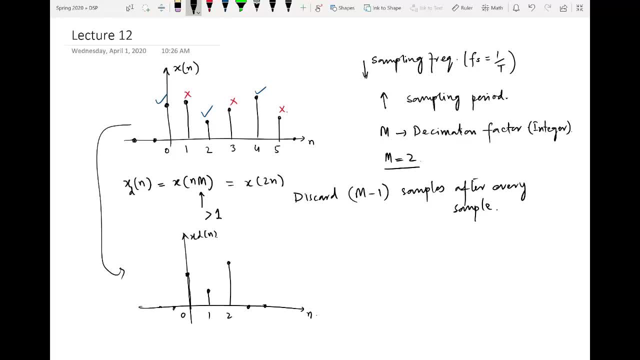 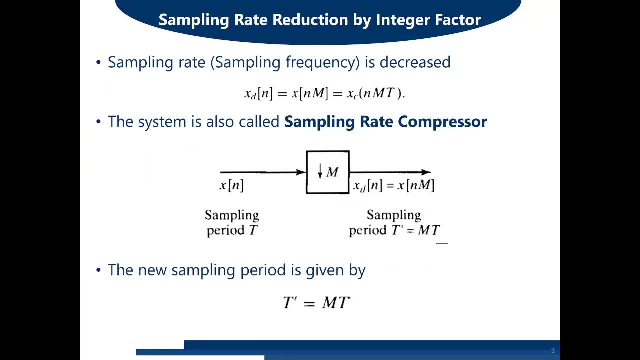 decreasing the number of samples, So we are decreasing the sampling rate. we are having less number of samples for a given time domain signal. So as a block level you can simply describe it as a sampling rate compressor, that if you have a time domain signal, 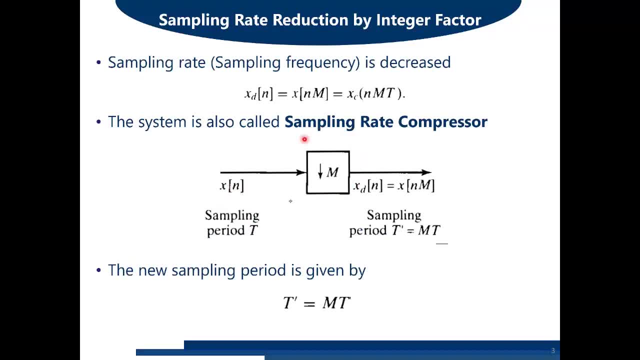 x of n and we usually denote the sampling rate reduction by this block or a circle, and this m is the decimation factor and this downward arrow is describing us that we are talking about decimation. In the interpolation the same arrow will be upward, So xd of n will be equal to x of nm. 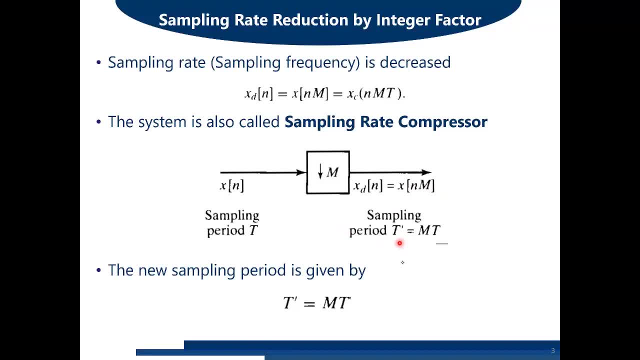 So the sampling period t prime, the new sampling period will be equal to m into capital T, because the sampling frequency is reduced by a factor of m, So sampling period will be increased by the same factor. So the new sampling period will be given by this one. and if you talk about the sampling 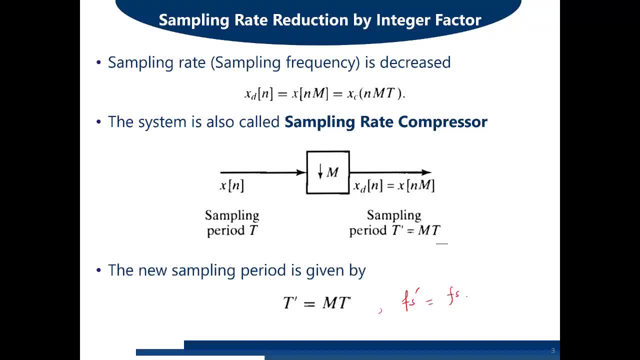 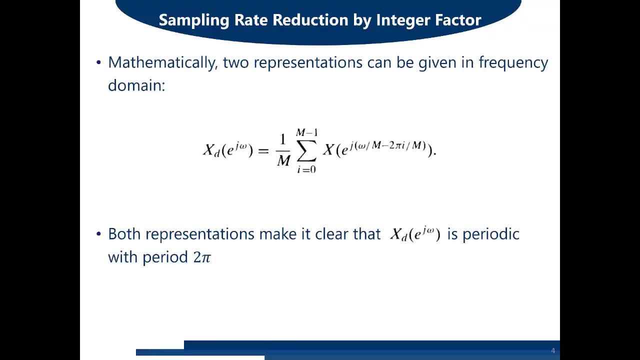 frequency, fs prime that will be equal to the original fs divided by the decimation factor. Okay, Now what we will happen in the frequency domain? This we have talked about the time domain. What will happen in the frequency domain? There is a complete derivation behind this, but 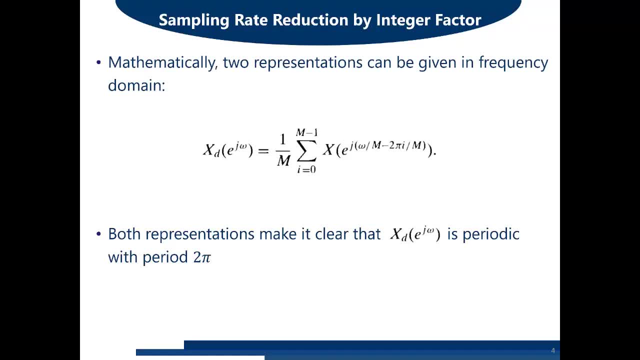 the end result I am going to discuss over here. just to give you a quick glimpse and what is happening in the frequency domain, I will show you, with the help of some magnitude responses, So you see the representation that will be the end result of DTFT. 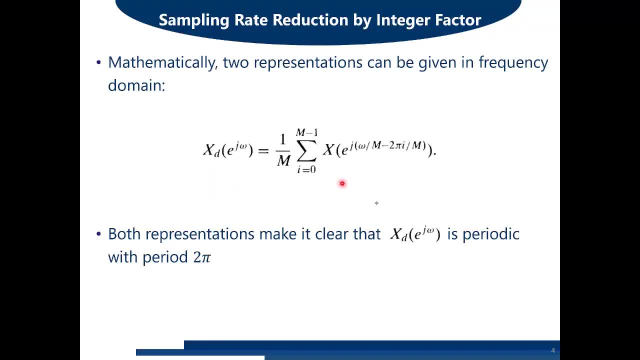 after performing decimation. that is shown by this particular equation Here. it is not very intuitive to understand this particular equation. I will explain this with the help of m is equal to 2, but the main point that you should keep in mind is that when we perform decimation, 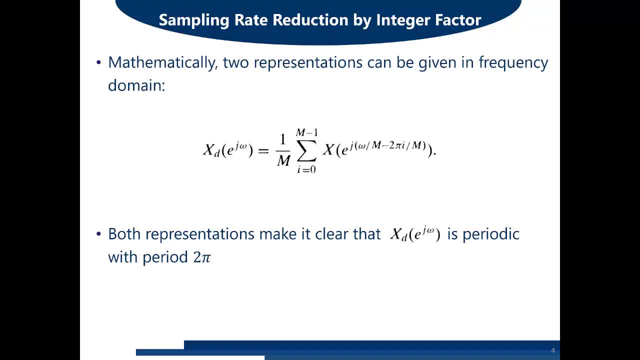 time domain signal is compressed and as a consequence, because time and frequency they are inverse of each other. So whenever a time domain signal is compressed, the corresponding frequency domain signal will be expanded. So the same concept will be applied over here. Während der Anpassung ist der Eininsky. 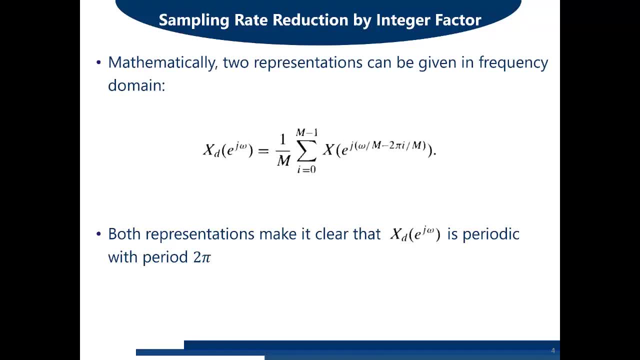 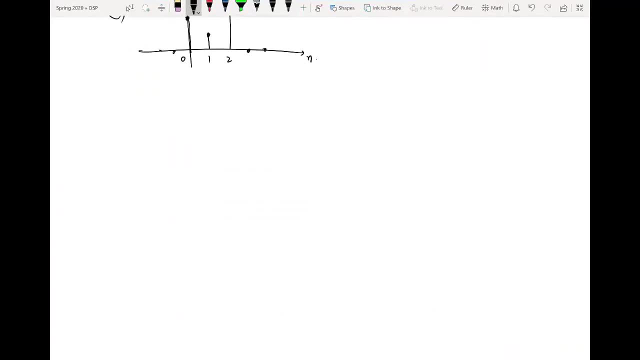 ist der Zeit auf der Prozession A, die Abrine, der Zwischen prends The time domain signal will be compressed. it will contain less number of samples and consequently its frequency domain plot or the magnitude response will be expanded by the same factor. Let me write the same equation. 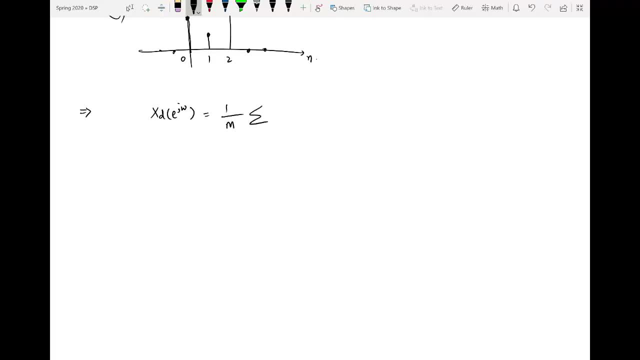 over here, and then I will explain to you with the help of m is equal to 2.. So it will become X B of e raised to power, j omega, the DTFT of the decimated signal, that will be 1 over m接имухa T. this will be 1 over m, With an equivalent. 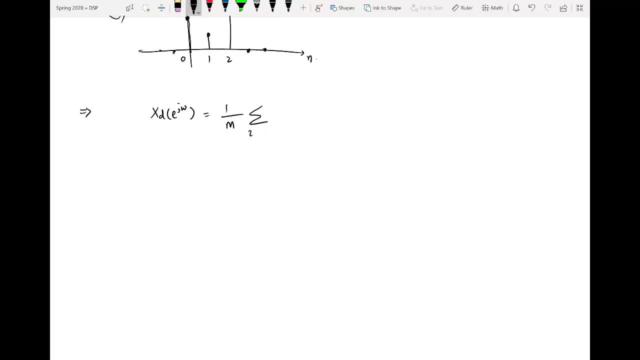 i is equal to 0 to m minus 1, x of e raised to power, j omega by m minus omega minus 2 pi i divided by m. So this is the equation that is giving you the DTFT of decimated signal. 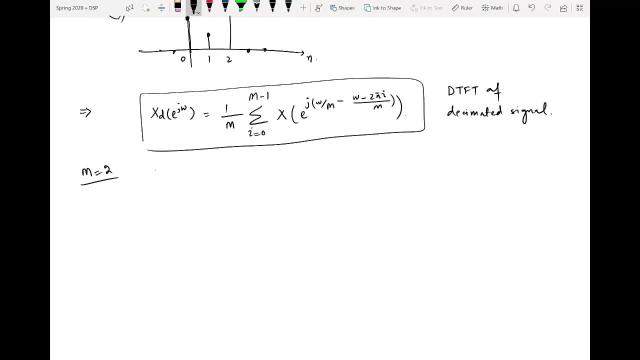 Now, if you take m is equal to 2, the same equation comes out to be x. e raised to power j, omega 1 over 2.. And the first term will be for i is equal to 0.. So it will be x of e raised to power j. 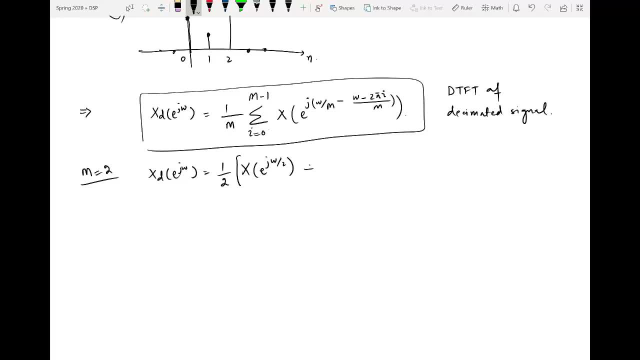 And the second term will be x of e raised to power j, omega by 2 minus omega minus 2 pi divided by 2.. So we will have two terms. So this equation is actually relating the DTFT before decimation to DTFT after decimation. 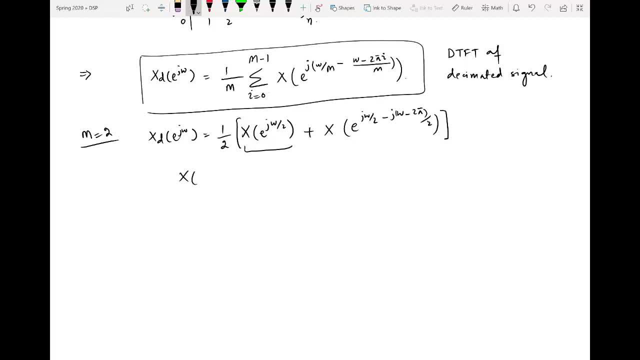 This one, x of e, raised to power j And omega, is basically DTFT before decimation. Now let us take an example How we can draw the DTFT by using this particular equation. Let us say we have, as you should know, that DTFT will always be periodic, with period 2 pi.